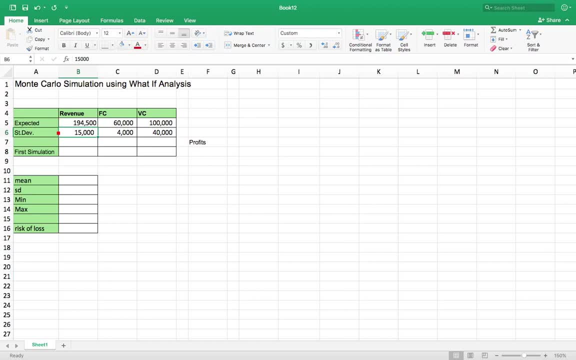 minus one standard deviation goes up 15, plus or minus two standard deviations would go up by 30. Your fixed costs are $60,000 with some standard deviation variation, and your variable costs $100,000.. Now this is assuming that there's a normal distribution around these inputs, which 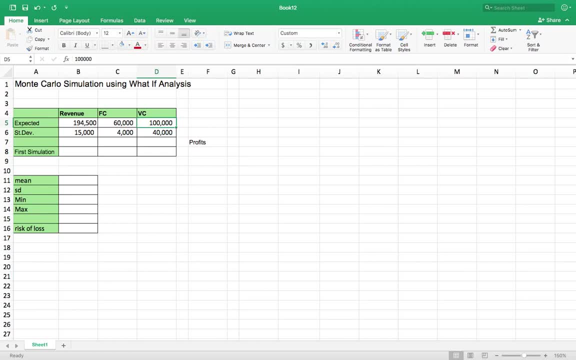 might not be the case. So if you do a simulation assuming normal distribution that is not normal distribution, your results will not be accurate. So let's assume these are normally distributed So you can use the in norm in to get a normal distribution from this revenue that has a $194,000 as. 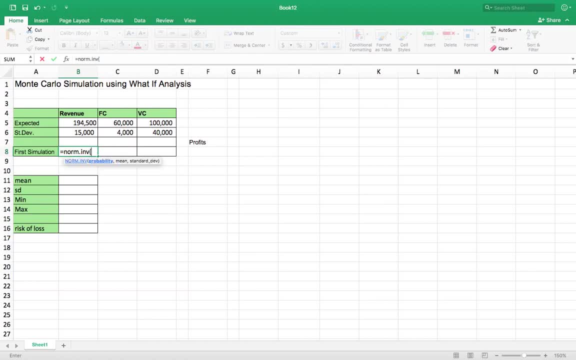 a mean and $15,000 as a standard deviation, And to randomly select from that you're going to use rand. You'll say: this is the mean comma, this is your standard deviation, Okay, And then you're going to drag that across to these three. There's a formula again. Now your profits are going. 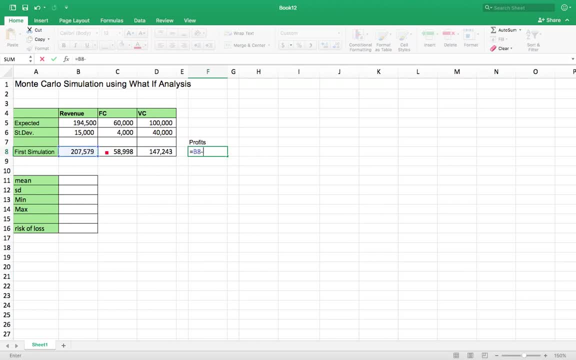 to be your revenue minus your fixed costs, minus your variable costs. And that right there is your first simulation of what your profits are going to be. I'm going to highlight that in yellow. So what we want to do is actually do a number of. 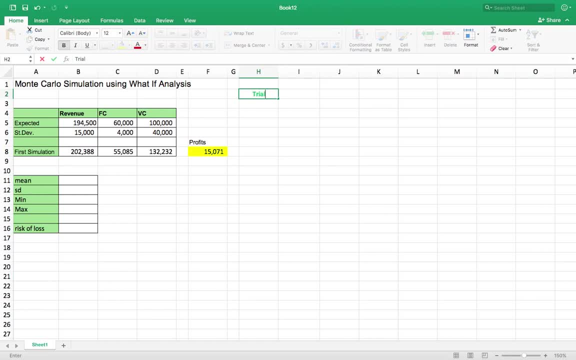 simulations and all I'm going to do, 500.. So there's the trial profits. So I'm going to grab the one here. I'm going to make a series by going to fill series one to 500 to column. Okay, Now, right here I'm going to. 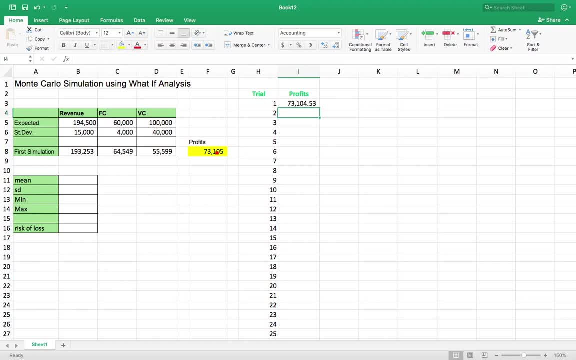 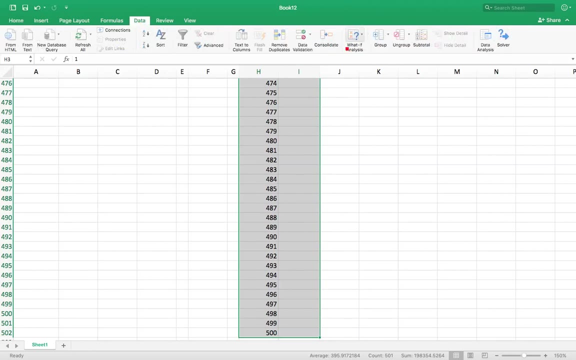 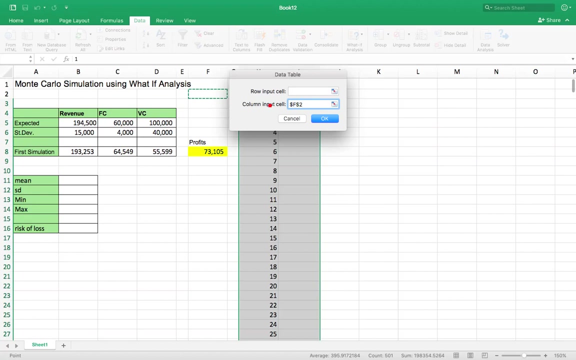 this profits. and now the highlight this table by hitting shift command down using a Mac we go to. what if analysis data table ignore row? just use cell input. choose any empty cell. it needs that cell to to work in and it should populate this. sometimes you have to wait for a moment, doesn't do? 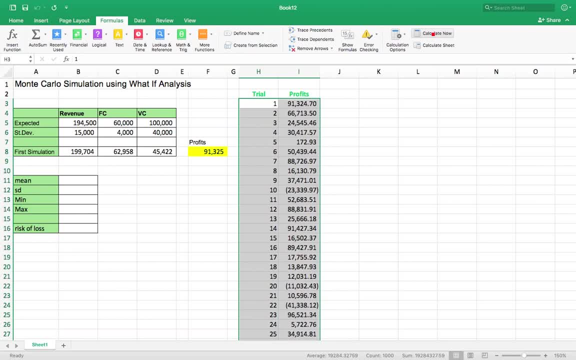 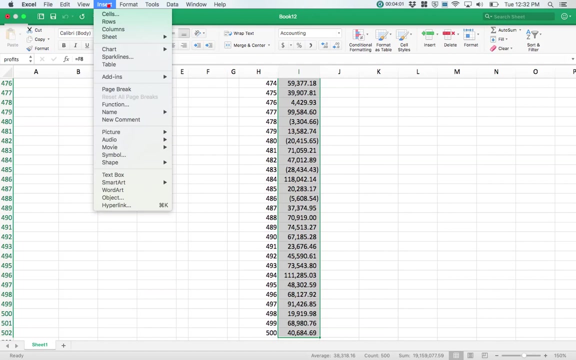 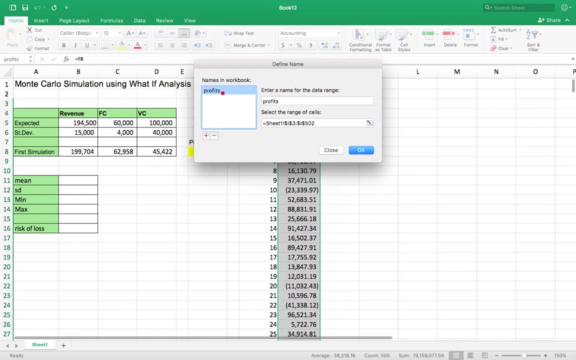 right away, go to formulas and calculate. now, there it is, populated, that row of profits. okay, so that's all well and good. so now what we might want to do is say, well, what's my average here, so let's name this, let's go into, you could insert name. I'm going to name this string of values, profits. I actually 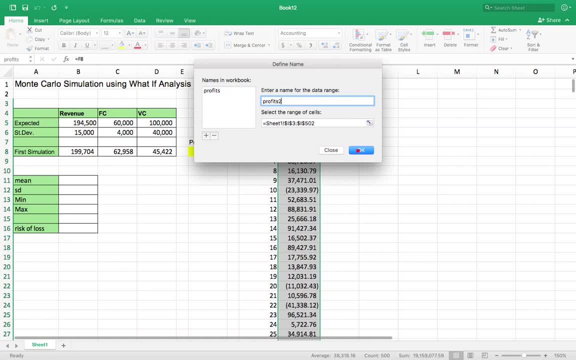 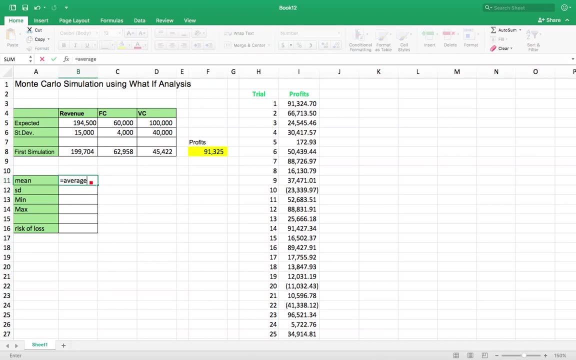 want to call it profits too, because it looks like there's already a profits in the workbook. well, that profits too. okay. so now you can say: mean equals average of profits to you saying it's a standard deviation profits too, it's a minimum, has going to be. 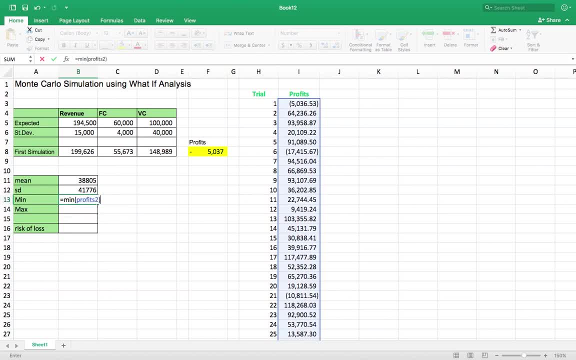 maximum. and then what I'd like to know is: what percentage of the time did it receive theAHT and what percentage of the time was it going to have a maximum of negative instead of positive? so, within a month, the average is going to be negative and this is going to be the. 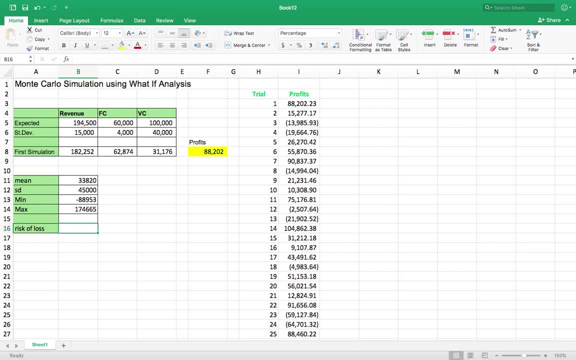 percentage of the time. is this going to give me negative profits? Am I going to lose money? So I'm going to say, count. if profits to comma in quotes is less than zero, I'm going to put that over 500.. Hopefully I did this correctly. Yeah it. 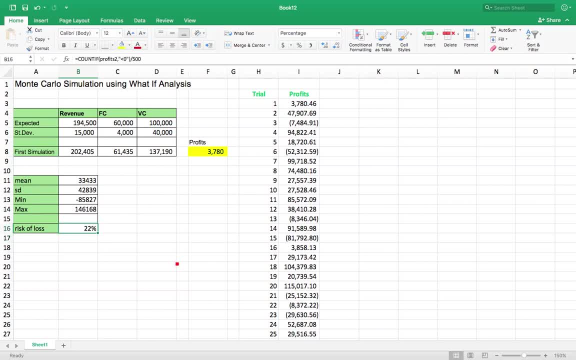 says about 22% of the time I'm going to be losing money with this particular setup, So you can keep recalculating that. Go into calculate now. You'll see there's a slight variation with all these random selections from these distributions. But you might want to use more trials. So what this is really doing. 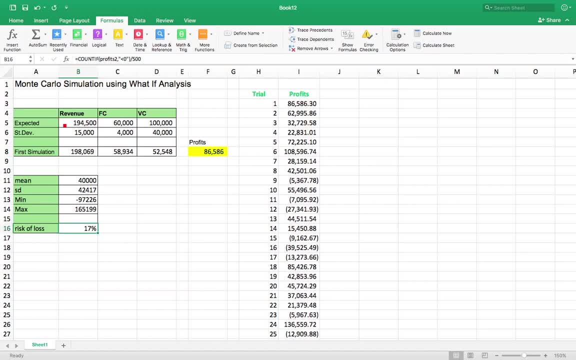